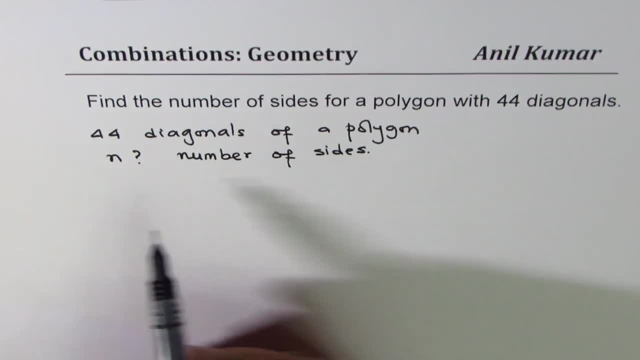 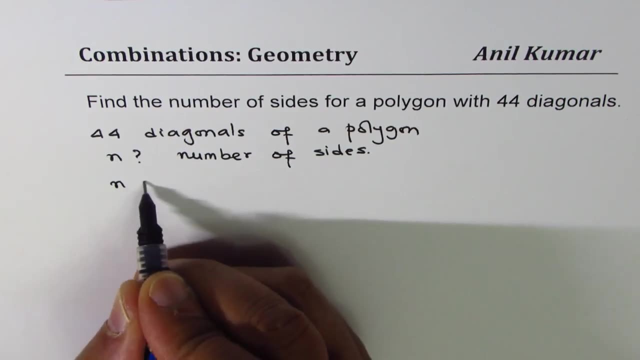 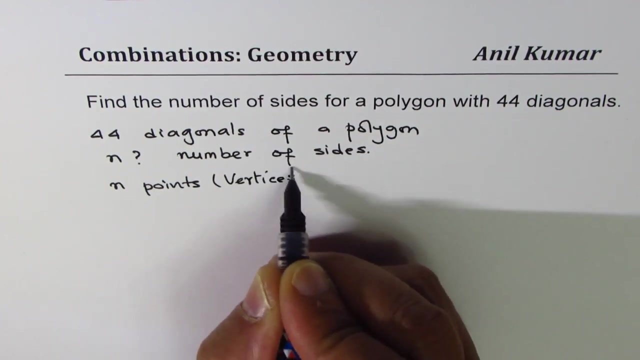 the number of sides of a polygon. Let us say the number of sides is n right. That means we have n points, which we call vertex right Or vertices right. So there are n vertices. If there are n vertices then we have to find the number of sides of a polygon. So we have 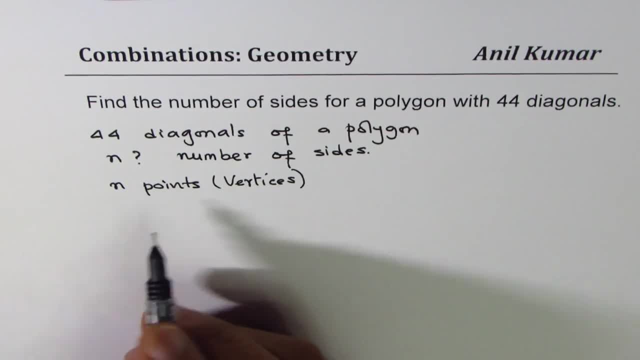 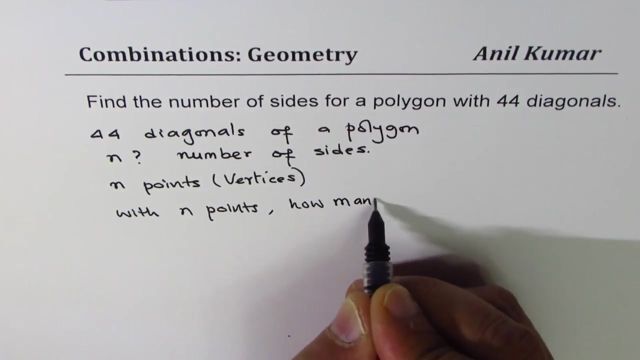 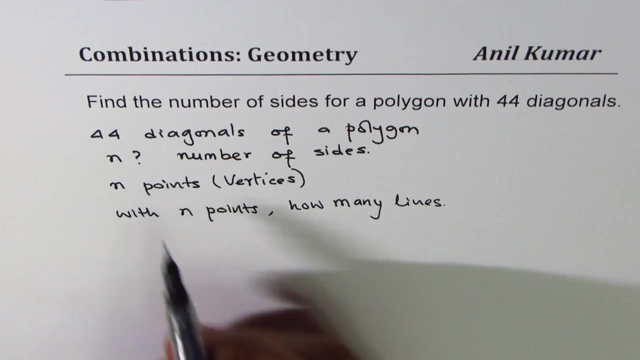 n points Maximum number of lines. how can you draw And how many can you draw? With n points, how many lines can be drawn? That is what you should think. How many lines can you draw? So for each line you need two points. So with n points we can draw nc2 lines Do. 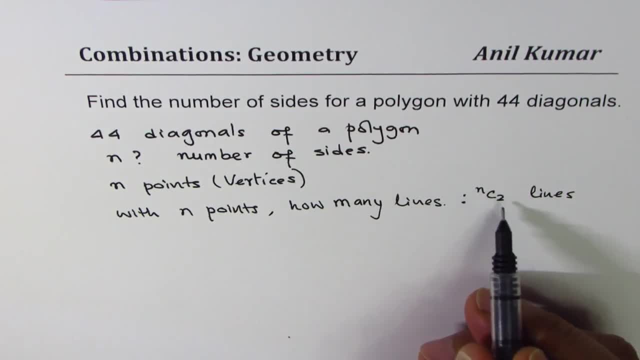 you see that? So you see that. So we can draw nc2 lines, Do you see that? So with n points, you can draw nc2 lines. Now, these are the total number of lines which can be drawn with n points. 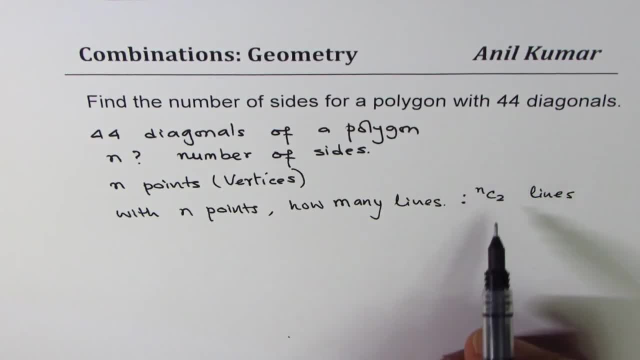 out of which how many are sides of polygons and how many are diagonals? Well, n are the number of sides And therefore the number of diagonal will be equal to nc2.. So how many NC2 total number of lines? take away n, which is the edges of the polygon, correct what we are given. 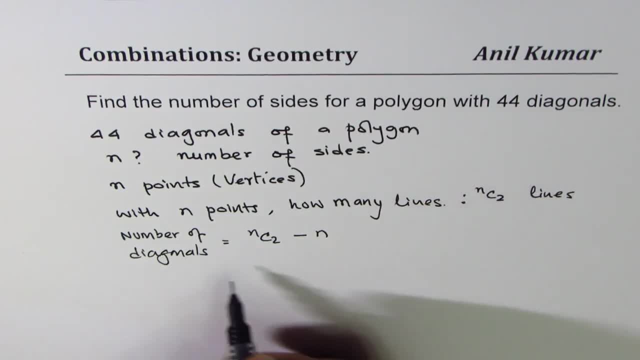 here is that there are 44 diagonals, so we could write this: as 44 is equals to NC2 minus n, right? so NC2 means n times n minus 1 divided by 2 minus. that is NC2, correct. n factorial divided by n minus. 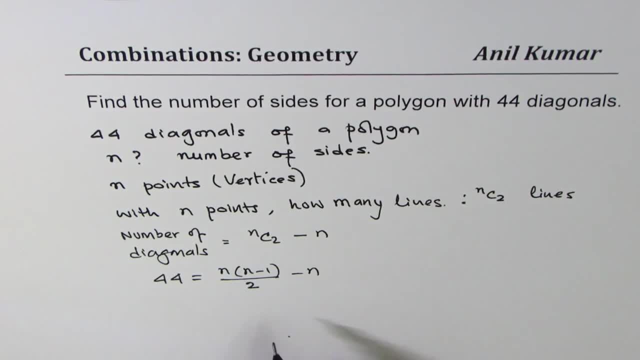 2 factorial divided by 2 factorial. that gives you this. now we can rearrange and solve for n. so what we have is 44 equals to n square minus n. taking common denominator of 2, we get minus 2n right. so let me say solve it on this side. so cross multiplies with 88 is: